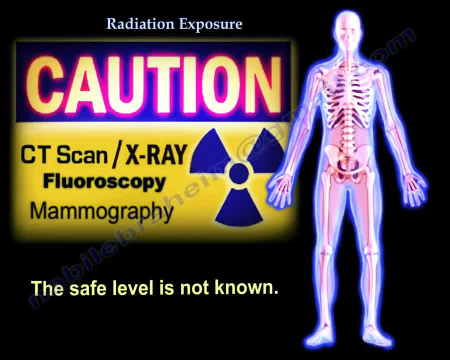 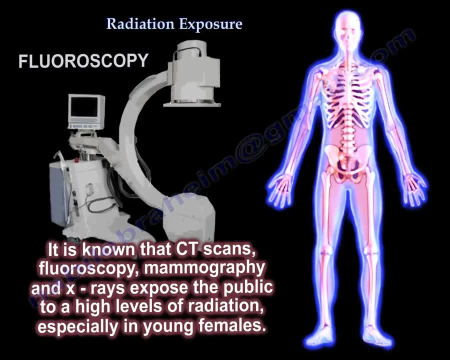 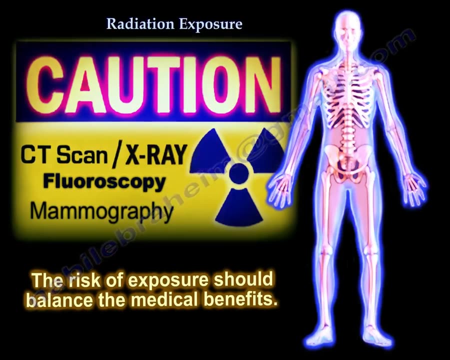 The safe level is not known. It is known that CT scans can cause cancer. CT scans, fluoroscopy, mammography and X-rays expose the public to a high level of radiation, especially in young females. The risk of exposure should balance the medical benefits. 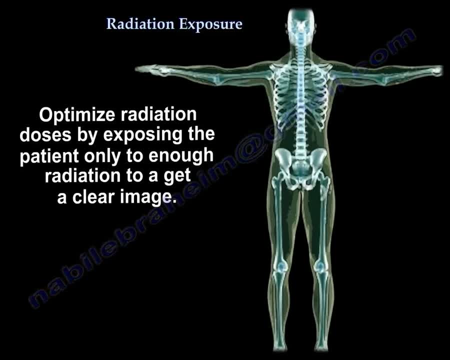 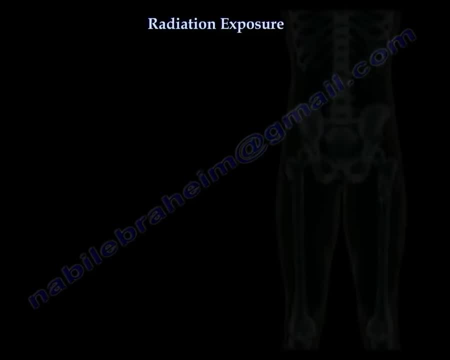 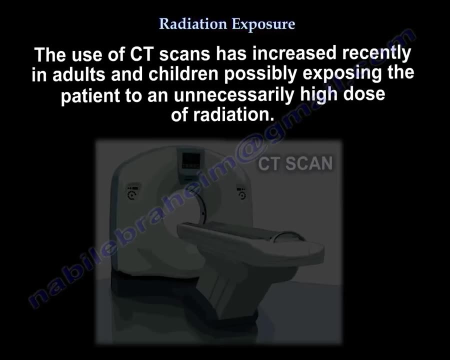 Optimize radiation doses by exposing the patient only to enough radiation to get a clear image. There is a growing concern about the risk of radiation exposure. There is a growing concern about the risk associated with giving a patient large doses of radiation. The use of CT scans has increased recently in adults and children, possibly exposing 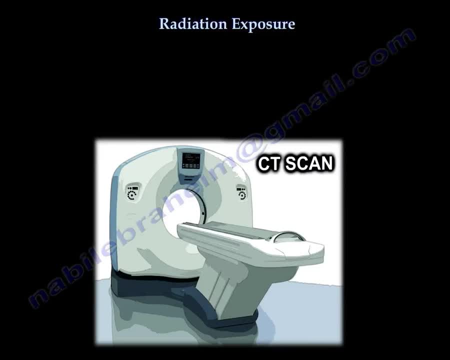 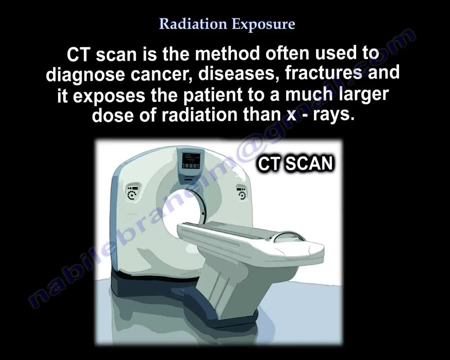 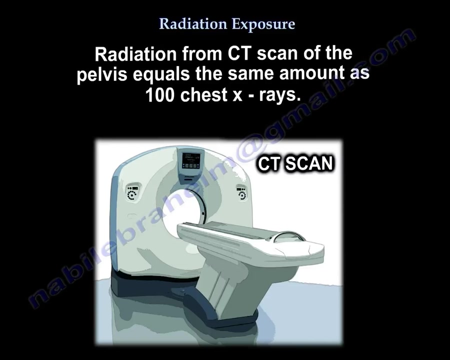 the patient to an unnecessary high dose of radiation. The CT scan is the method most often used to diagnose cancer, diseases, fractures, and it exposes the patient to a much larger dose of radiation than X-rays. Radiation from CT scan of the pelvis equals the same amount as 100 chest X-rays. Children. 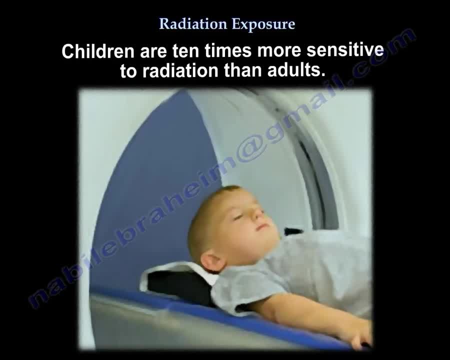 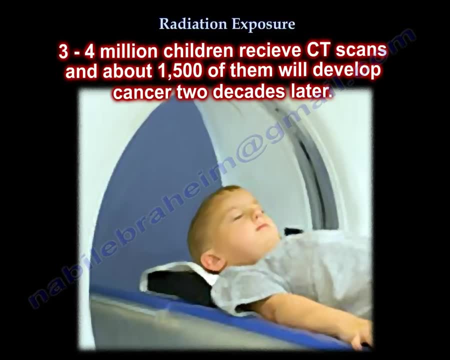 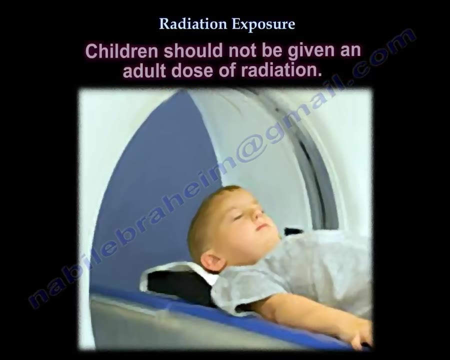 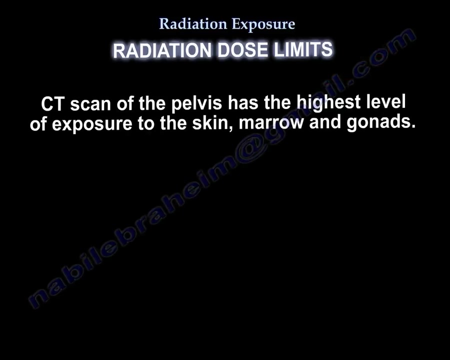 are 10 times more sensitive to radiation than X-rays. 3 to 4 million children receive CT scans and about 1,500 of them will develop cancer two decades later. Children should not be given an adult dose of radiation. Radiation Dose Limits. 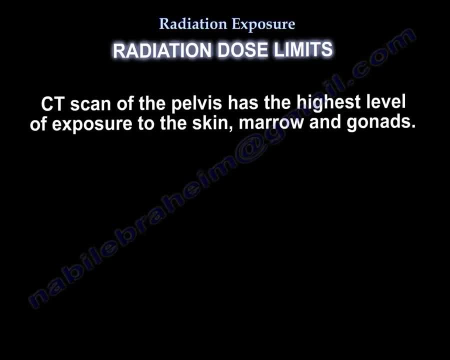 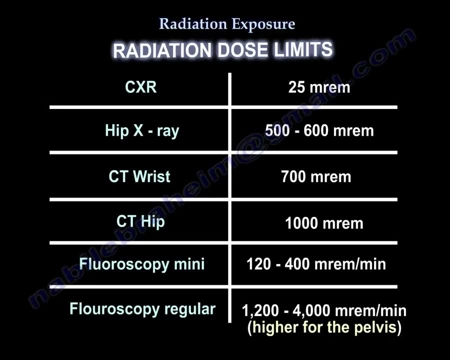 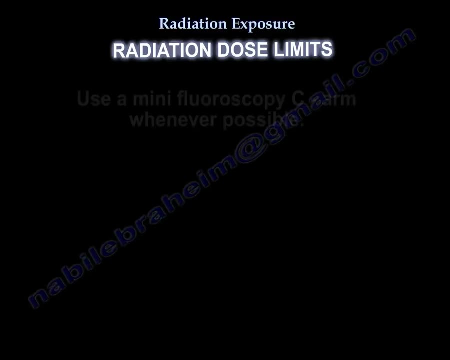 CT scan of the pelvis has the highest level of exposure to the skin, marrow and gonads And you're going to want to use a small size, small size CT scan unless your patient has a large enough amount of radiation in their blood. 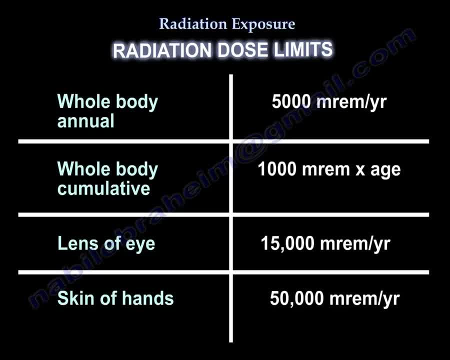 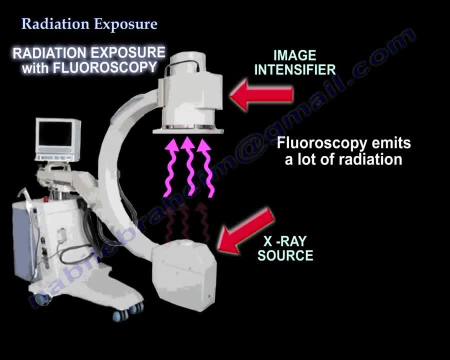 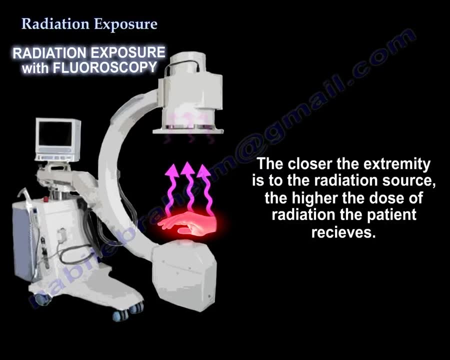 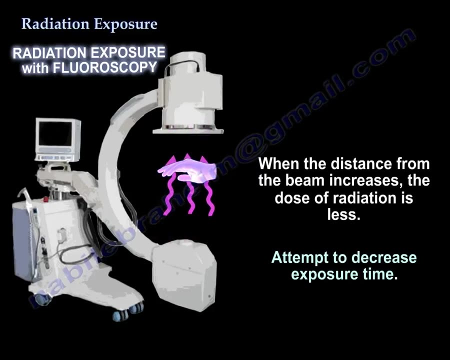 Truncating. Truncating Fluoroscopy emits a lot of radiation. The closer the extremity is to the radiation source, the higher the dose of radiation the patient receives. When the distance from the beam increases, the dose of radiation is less. 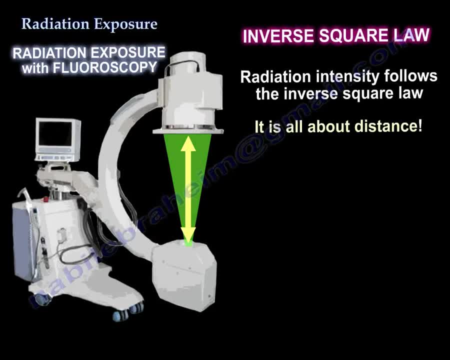 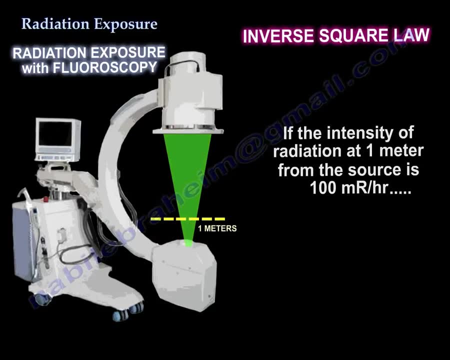 Radiation intensity follows the inverse square law. It is all about distance. If the intensity of radiation at 1 meter from the source is 100 millirenkin per hour, then the intensity of radiation at 2 meters from the source is 1, fourth or 25 millirenkin per hour in same unit area. 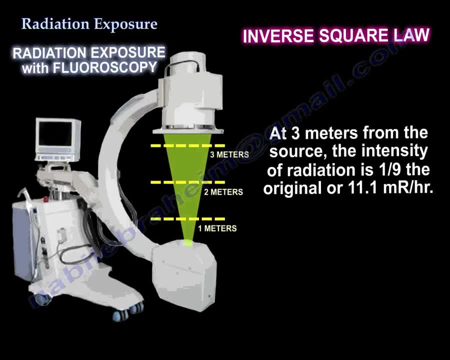 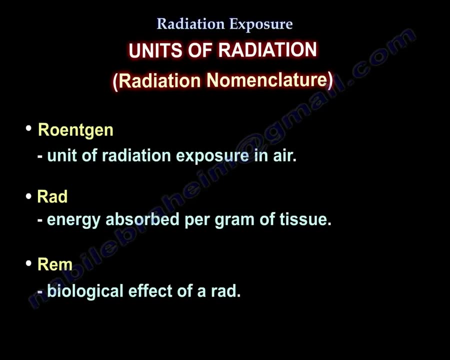 At 3 meters from the source, the intensity of radiation is 1 ninth the original, or 11.1 millirenkin per hour. At 3 meters from the source, the intensity of radiation at 1 meter from the source is 1 ninth the original, or 11.1 millirenkin per hour in same unit area. 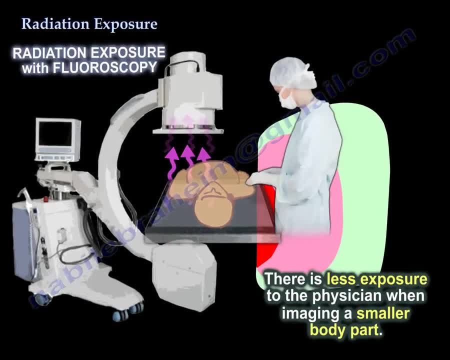 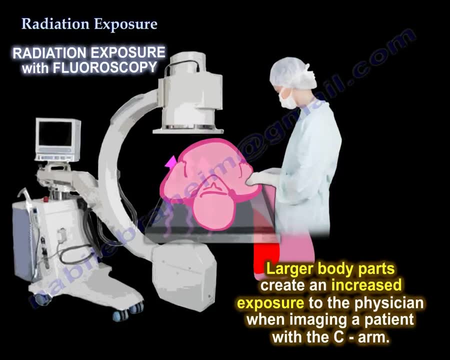 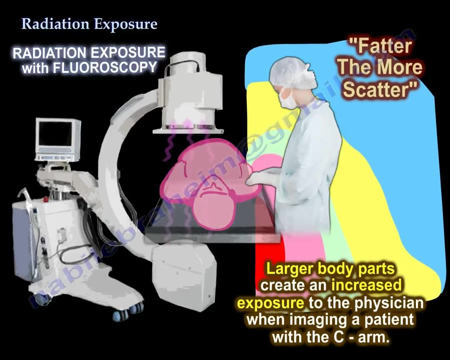 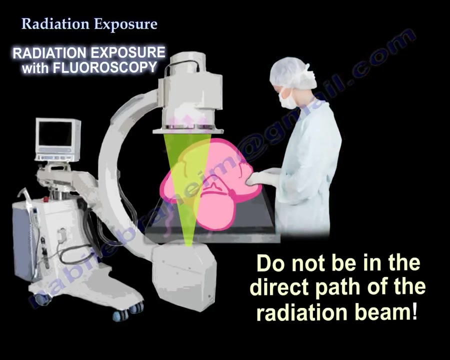 There is less exposure to the physician when imaging a smaller body part. Larger body parts create an increased exposure to the physician when imaging a patient with the CR. Do not be in the direct path of the radiation beam. Radiation protection is of importance with monitoring, shielding and position. 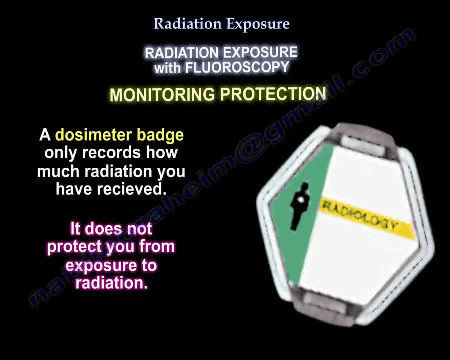 Monitoring protection should be used with a desometer badge. A desometer badge only records how much radiation you have received. It does not protect you from exposure to radiation. Shielding protection of fluoroscopy radiation, Lead gowns and aprons work to stop exposure. 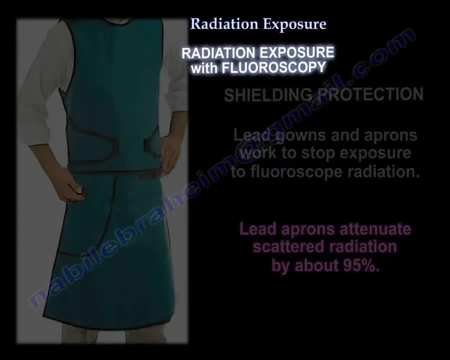 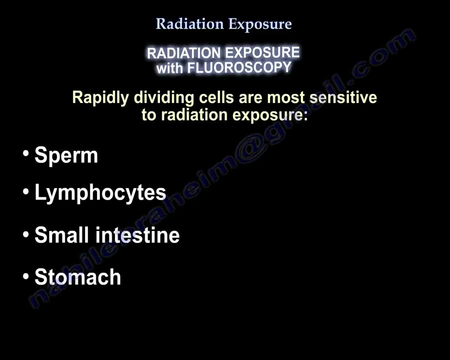 Lead gowns and aprons attenuate scattered radiation by about 95%. Rapidly dividing cells are most sensitive to radiation exposure, such as sperm, lymphocytes, the small intestines and stomach. Radiation damage seldom appears at the time of irradiation. 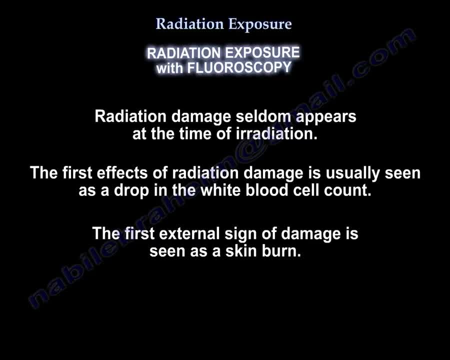 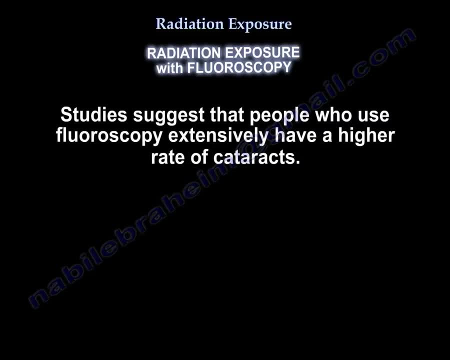 The first effects of radiation damage is usually seen as a drop in the white blood cell count. The first external sign of damage is seen as a skin burn. Studies suggest that people who use fluoroscopy extensively have a higher rate of cataracts.